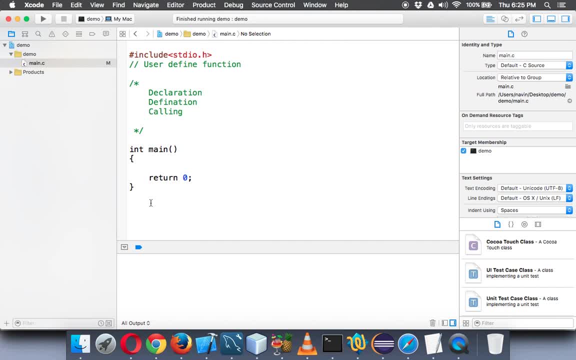 now, when you say you want to create a user defined function, so the the, what you say, the steps or the syntax for a function will be: you have to define the return type of a function. now your function might return int, it might return float, or it may it will return nothing. so if your 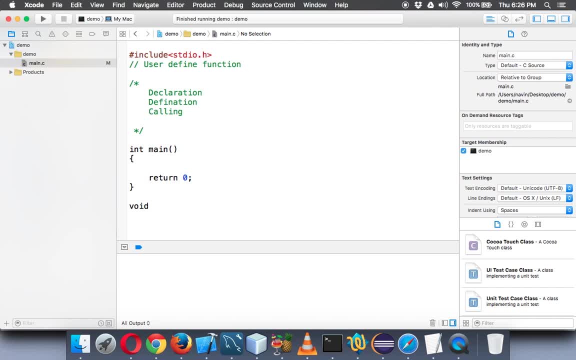 if your function doesn't return anything, we'll simply write void and we have to define a function name. so, using a function which is called a show, so you can name any fun, you can have any name, provided it follows the rule. uh, it cannot be. it cannot start with special symbols. you cannot use. 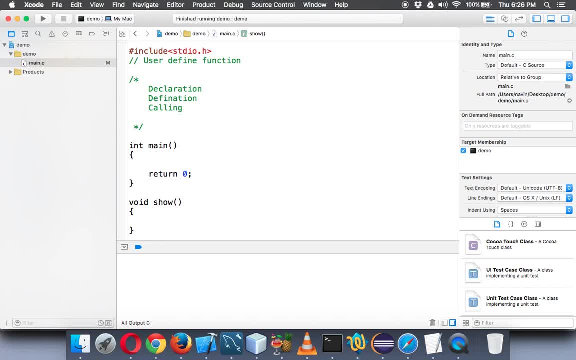 special symbols for functions. uh, so you have to give a character string here now. uh, you can, you're, can, make it work. okay, so you have to. let's say you want to print something. so let's say you want to print high. so this is what your function is doing, right? so 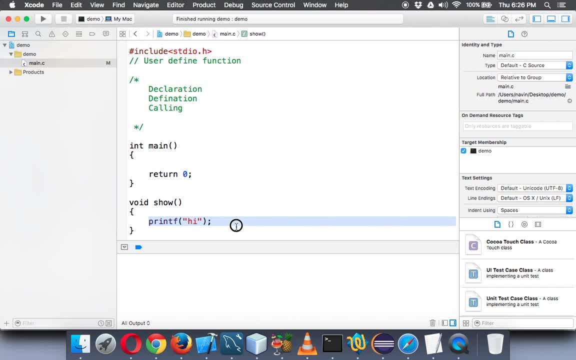 your, your function show is printing high. but this step from here to here, this is call as definition. but we are missing a part. we are missing declaration, now way to define. so before the main function or before the before any function, you have to say: you have to define this, you have to declare this function. how to declare? 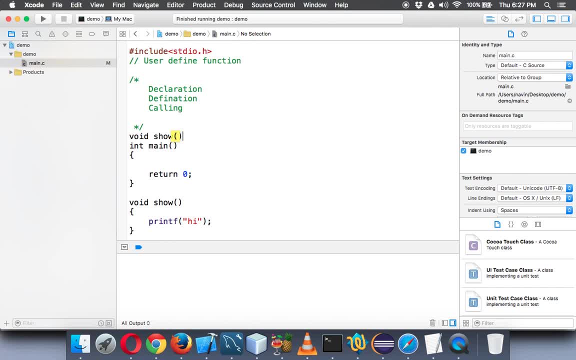 so you have to again mention the event type and you have to say show, but the difference will be in definition. you have to use curly brackets in declaration. you have to mention a semicolon, because you are not defining it, you are declaring it okay. so this is your first step, declaring the method, and it is your. 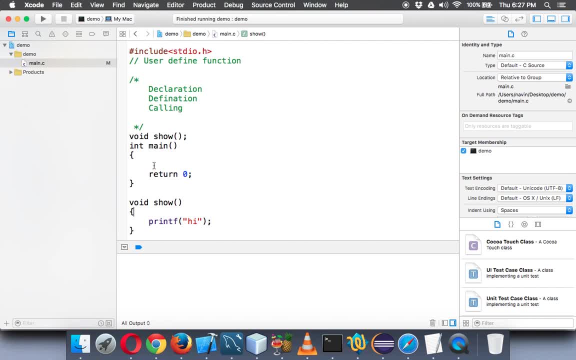 second step here to define it. now, once you're done with the first two step, we have to call this function and how to call. we have to use a function name and a semicolon. so in you calling, we don't if we don't mention the written type, and that's what the 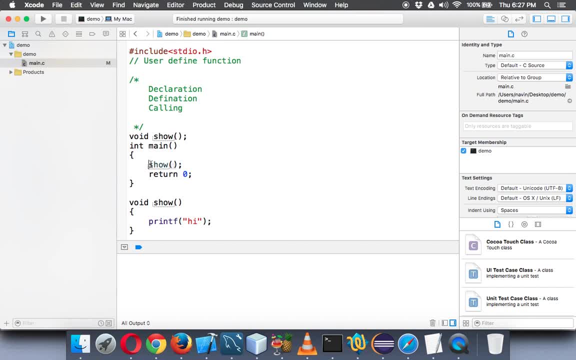 main difference between declaration and calling. so make sure you don't define, you don't mention the written type. okay, so this is declaration, this is the different definition and this is calling. so if I run this, you can see there's output call as high. okay, let me just print on a new line, run and you can see.